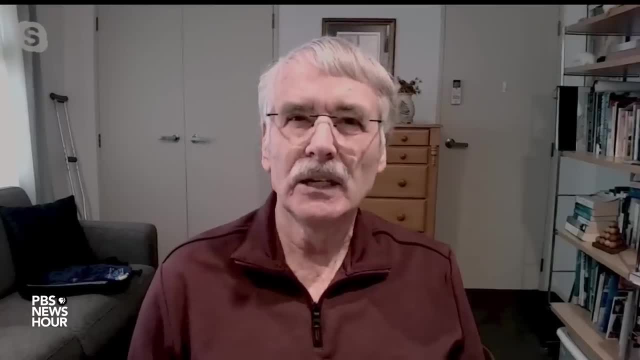 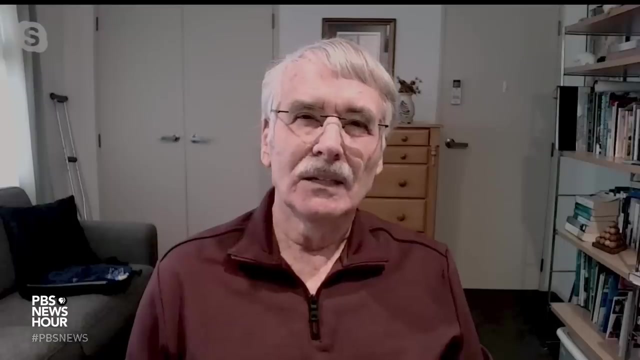 and Ecuador. that is disrupting the fisheries and so on there And it has warmed across all of that sector there so that the oceans, the sea surface temperature now as a whole is the warmest on record and has been April, May and into June. 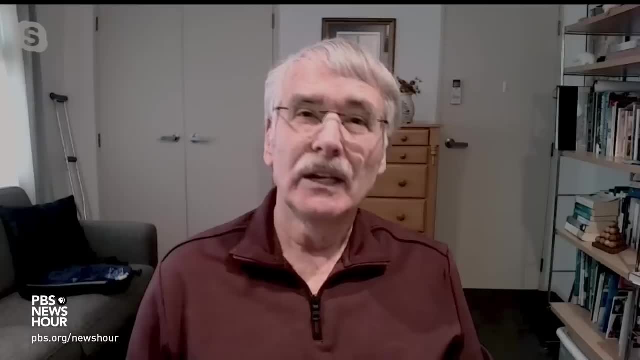 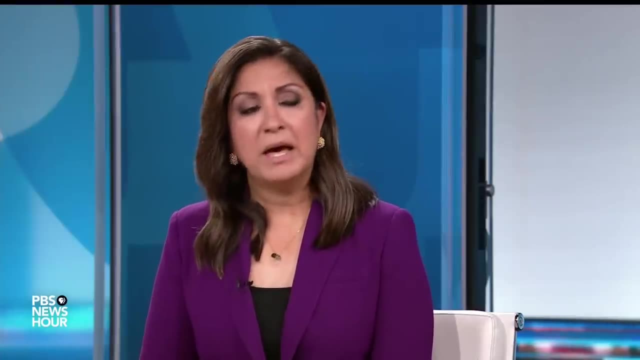 And we're running two-tenths of a degree Celsius above anything prior to that and substantially above the long-term average AMNA NAWAZ. So let's talk about one of the impacts of that. What do those two conditions coming together mean right now, as we're moving into hurricane season in particular, where 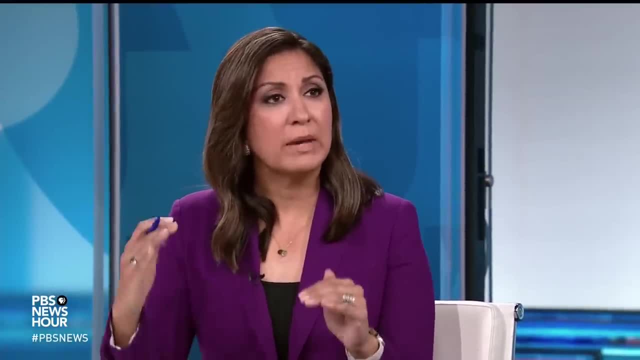 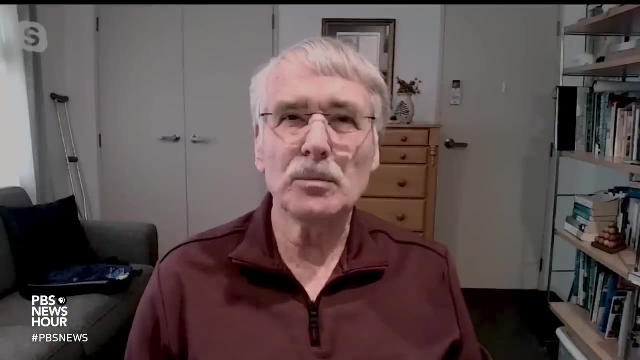 you have an El Nino event is under way and the warming of the ocean temperatures. What does that mean, DR ANTHONY FAUCI? Yes, it means that, along with the general weather that goes on, there are hot spots in the ocean that are becoming increasingly. 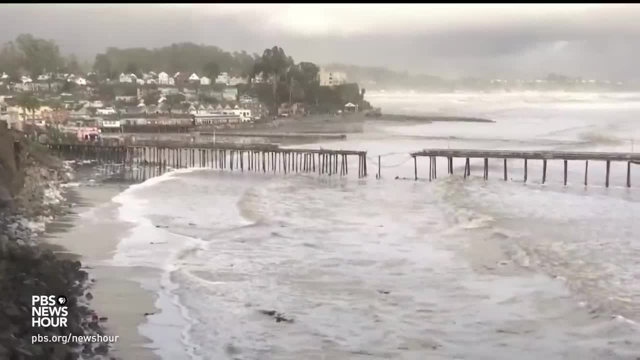 intense and frequent, And those hot spots tend to attract a lot of weather activity above the ocean. DR ANTHONY FAUCI, Yes, DR ANTHONY FAUCI, Yes, DR ANTHONY FAUCI, And so you know there's a lot of them. 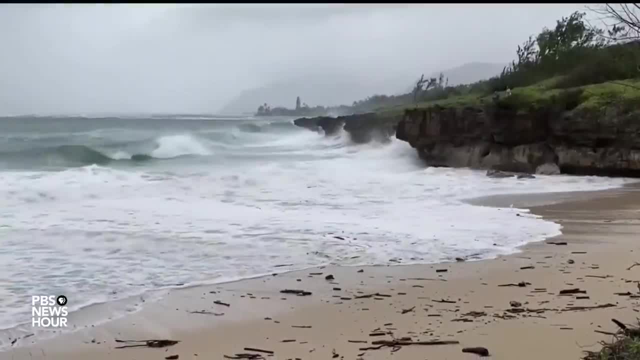 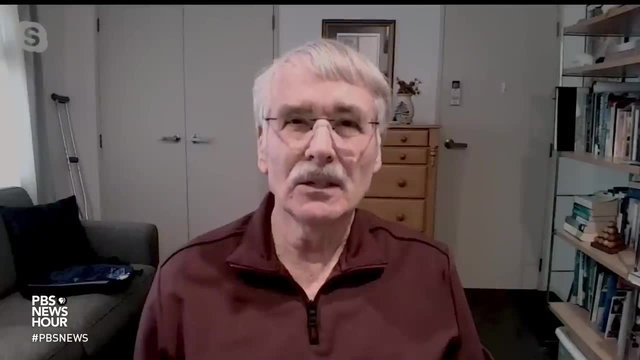 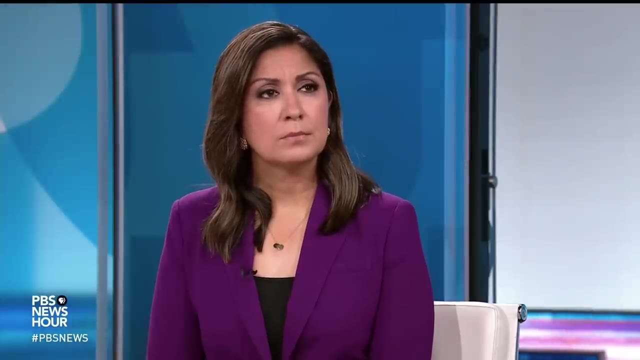 convection of different kinds, small-scale storms. They intensify tropical cyclones or hurricanes that are in that area. They move around naturally, And so it's a little difficult to say exactly where these spots are going to be, But the fact that they are occurring. 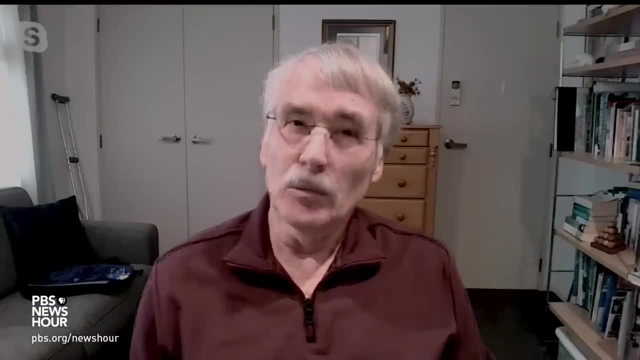 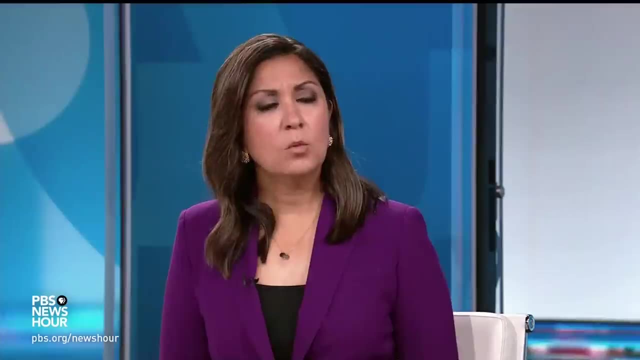 more and more is a part of this overall global warming signature that we have, And they have real consequences in many ways. AMNA NAWAZ, What about the ocean? What is the impact of those warmer waters on aquatic life? I'm sure you saw there were. 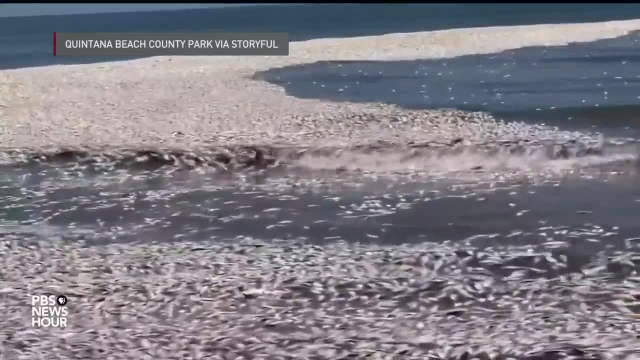 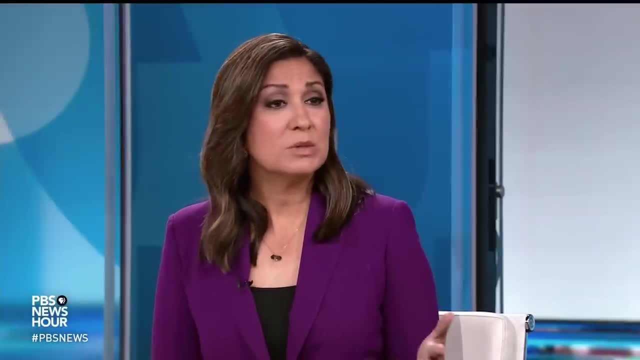 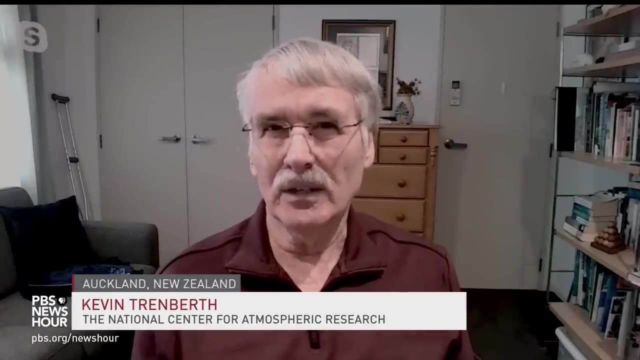 some pictures that got a lot of attention recently, showing thousands of dead fish washing ashore along the Texas Gulf Coast in recent days, How much of that is attributed to those warmer waters, DR ANTHONY FAUCI? Well, with global warming, the, you know, over 90 percent of the excess. 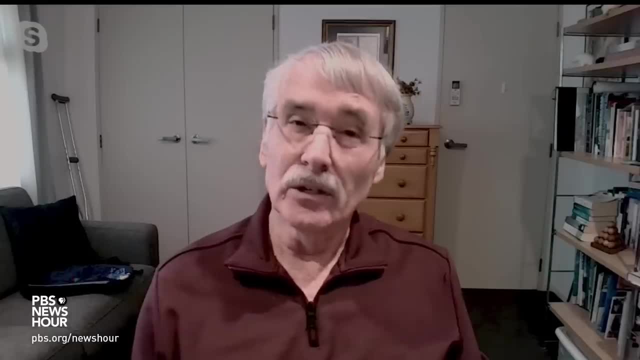 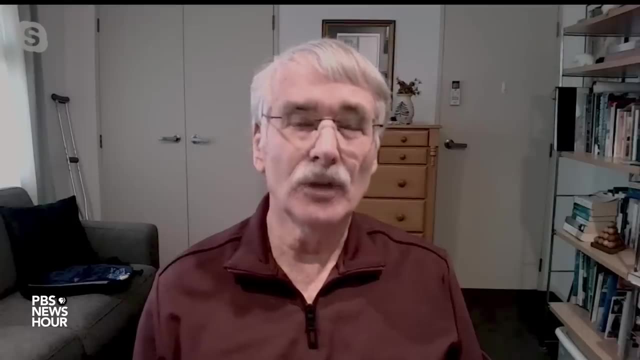 energy which is being generated every day goes into the oceans, And in the oceans it warms from the top. DR ANTHONY FAUCI, That means that we're sitting in a very stable configuration, DR ANTHONY FAUCI. So one of the things we have been able to document is that the oceans 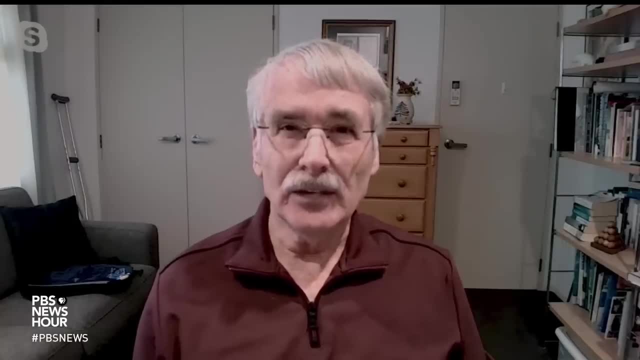 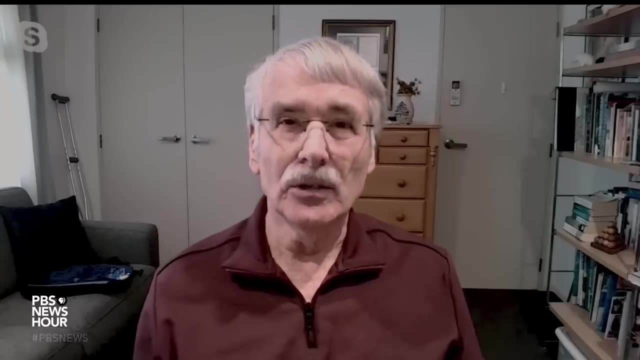 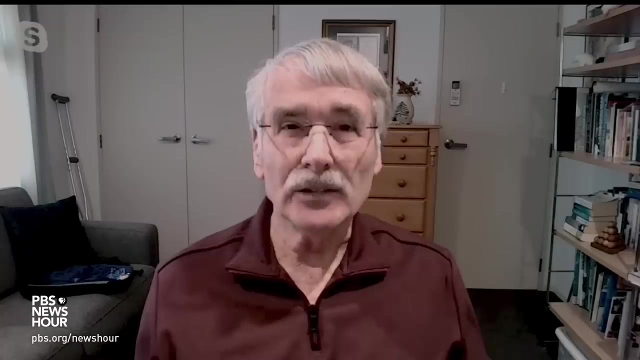 are becoming more stratified. That means that the natural exchanges of air of all kinds, including carbon dioxide and oxygen, going into the ocean are a bit less than they used to be Now. in general, this is overcome by wave action, so by all sorts of disturbance. 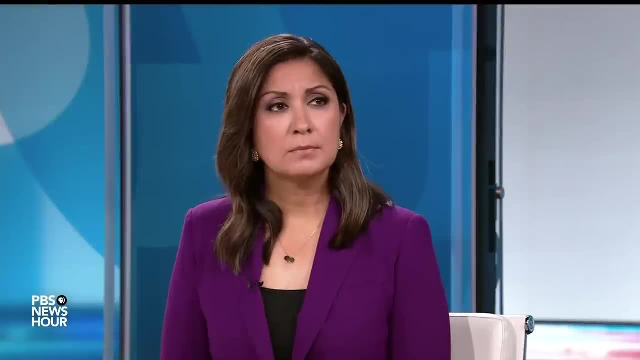 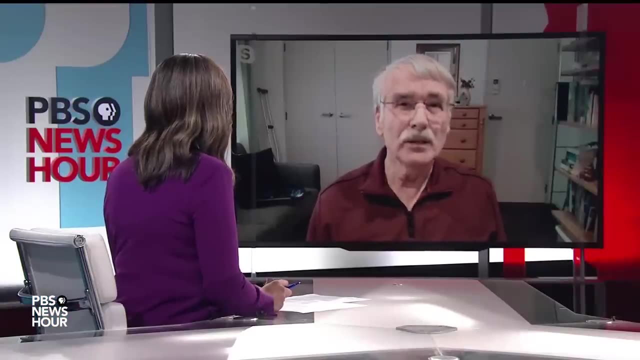 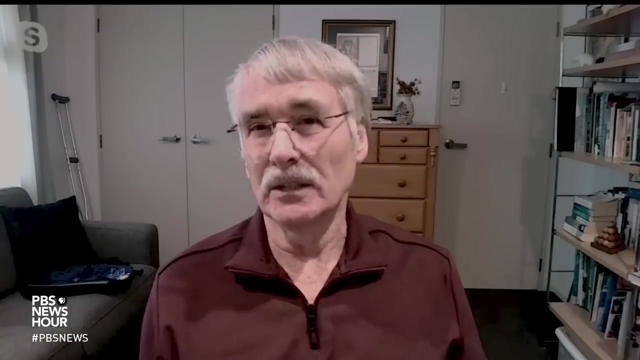 disturbances in the atmosphere, But in conditions where there are no waves, where there's no wind to speak of, and I believe that's what happened in the Gulf. In the Gulf it can also be complicated by nutrient runoff, some pollution in the Gulf itself. Those 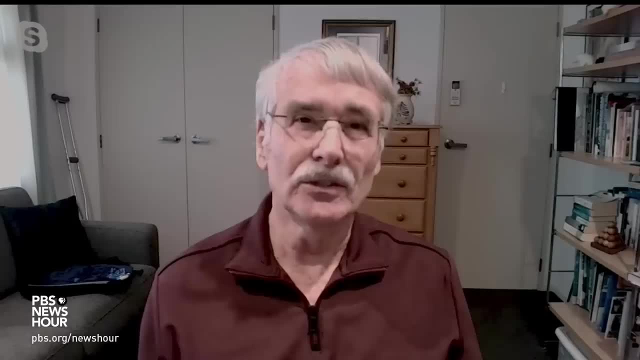 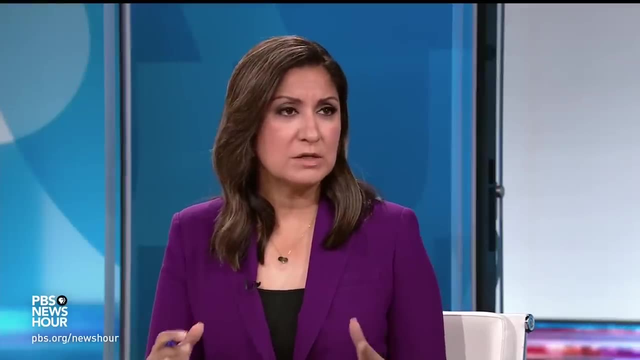 conditions come together and create anoxic conditions, no oxygen for the fish, And so you have this big die-off AMNA NAWAZ. So, Kevin, big picture. when people see these increases in temperatures and it catches their attention, causes concerns. they see global sea and air temperatures are. 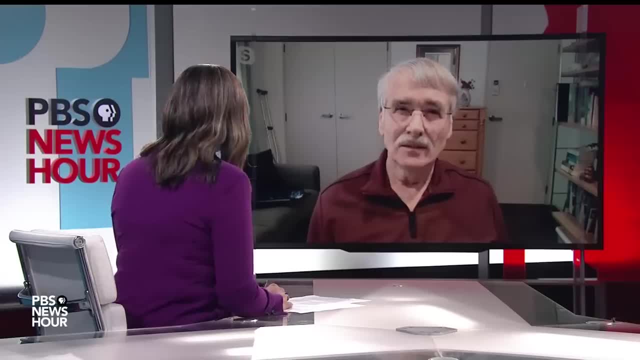 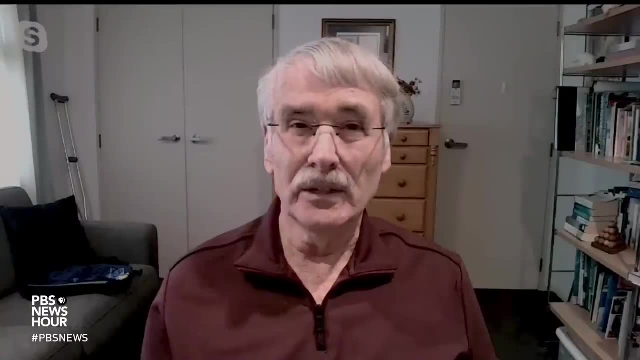 at record highs for this time of year. What should they understand about that? How much of that is attributed to climate change And do we expect that increase to continue? KEVIN HARTMANN, The first part of the year is going to hold. 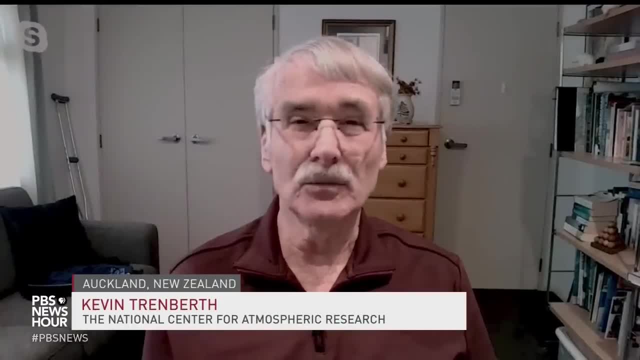 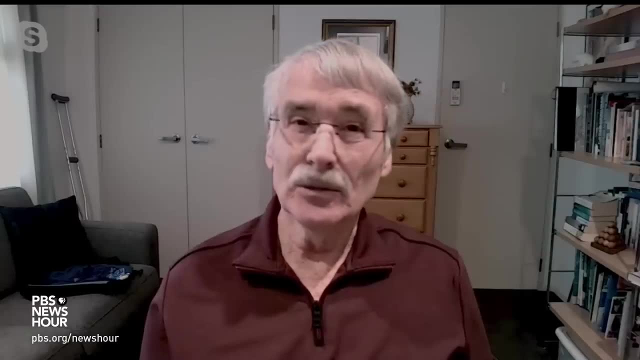 it down. So 2023 may not quite be the warmest year on record At the moment. I think that's really held by 2020.. But it will be close and it could well be. But 2024 certainly is looking as though it's. 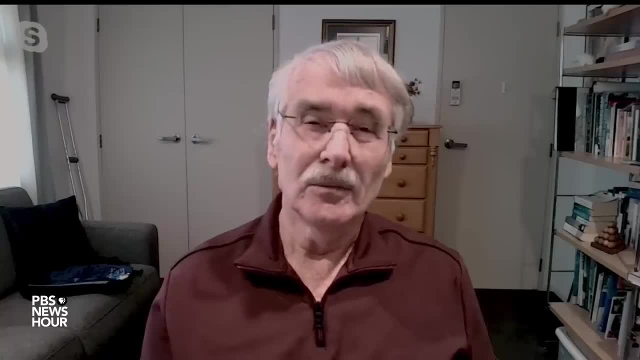 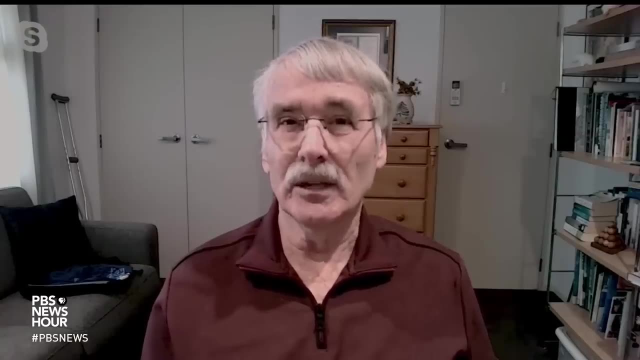 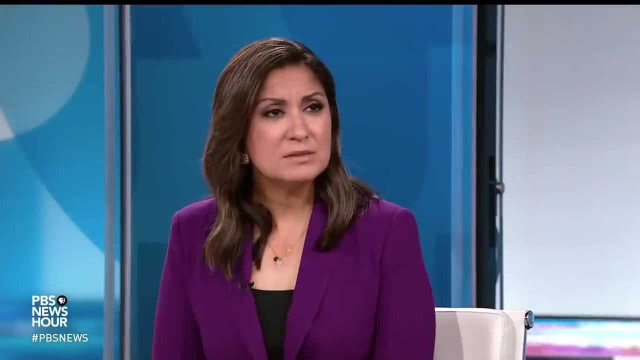 going to be the warmest year on record, And part of this is El Nino, but certainly the relentless increases in temperatures around the world are related to the global warming problem that we have the climate change AMNA NAWAZ, And do these increases say to you in any way? 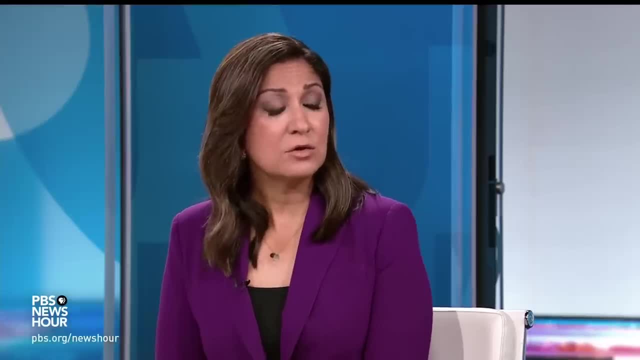 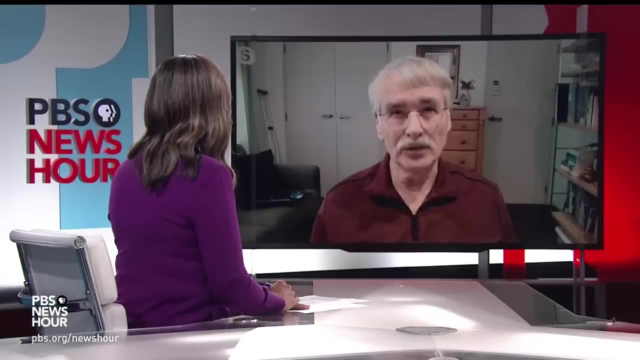 that the rate of climate change is accelerating. That's the other concern, right, MICHAEL FRIEDMAN? It is indeed the case that the amount of carbon dioxide in the atmosphere continues to go up, and it continues to go up at close. 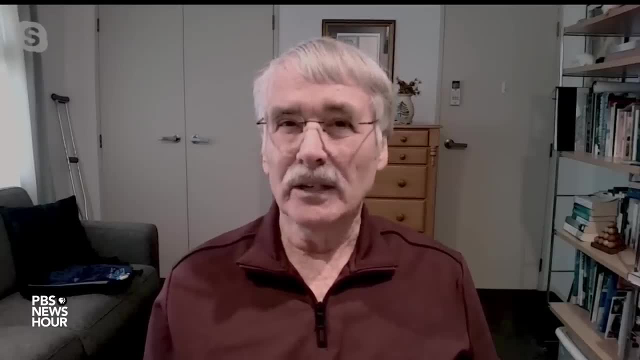 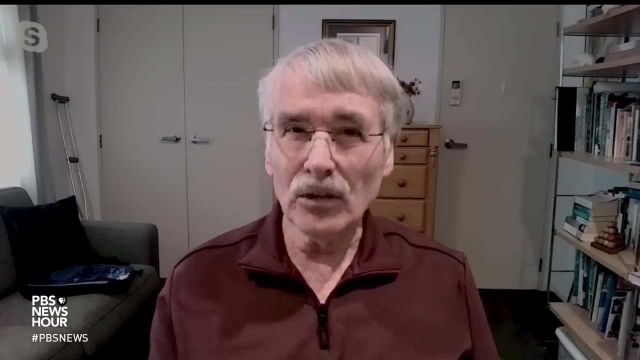 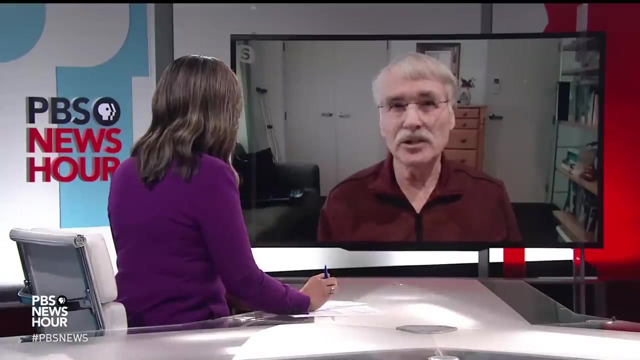 to record levels. There's been very little indication that all of the actions that governments and people around the world are taking is really knocking back the amount of emissions of carbon dioxide into the atmosphere. This is really the bottom line as to how the atmosphere is changing And carbon dioxide 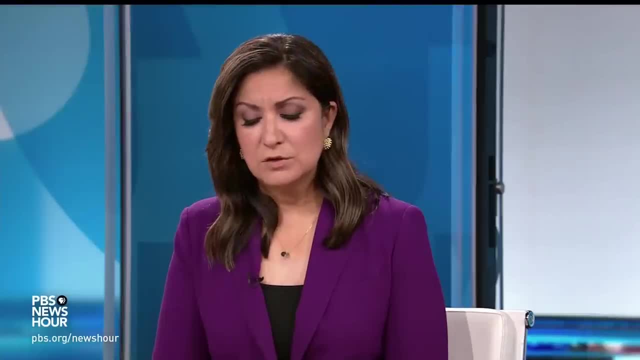